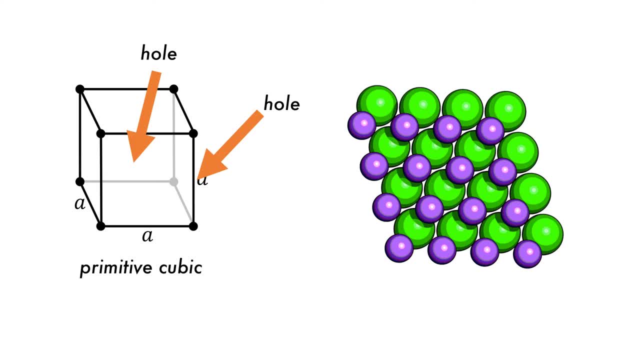 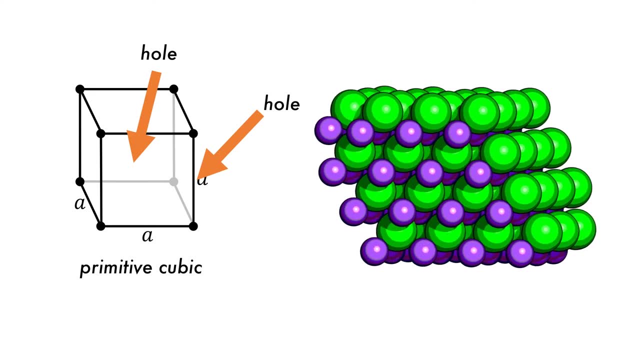 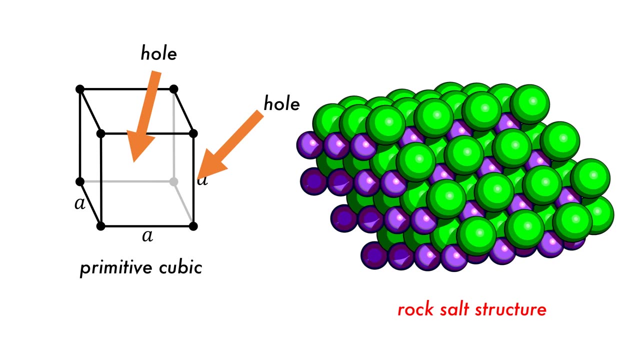 charge interactions. The combination of smaller cation and larger anion also increases packing efficiency. This can be seen in sodium chloride, where the smaller sodium ions sit in the spaces between the chloride ions. This is often referred to as the rock-solid structure. 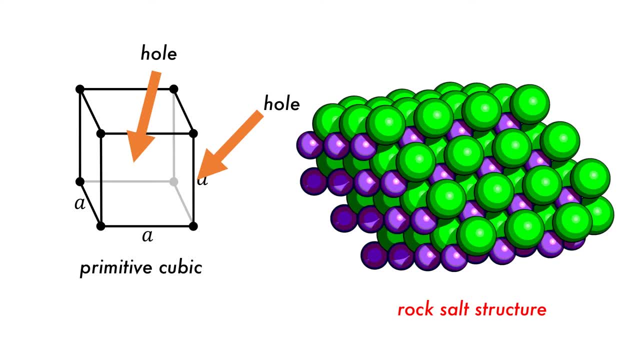 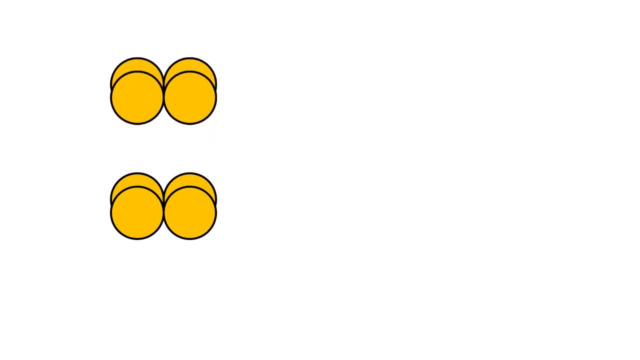 and is similar to, but not the same as, a BCC structure. Let's start with the simple cubic hole. If we explode a primitive cubic, we can see that there is space for a particle in the center of four particles. This is the simple cubic hole. This is similar to the BCC structure. 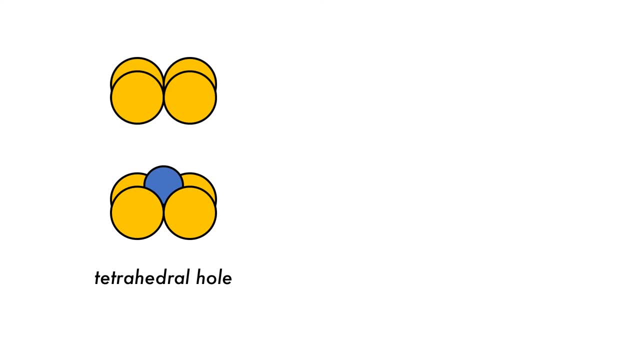 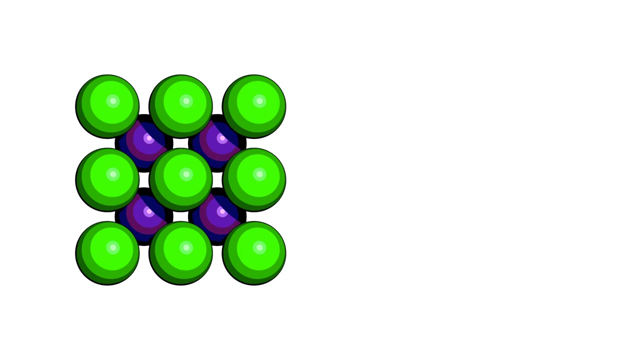 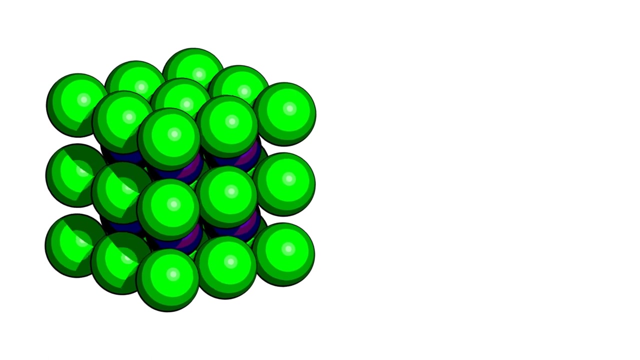 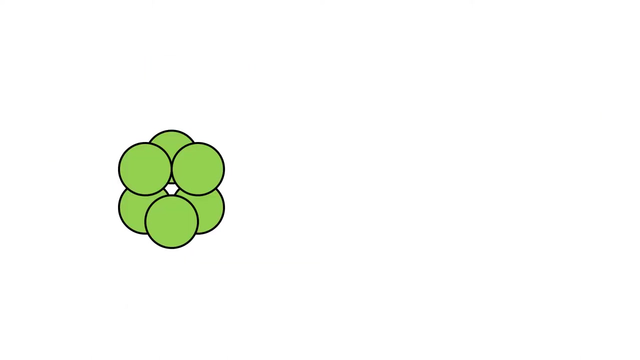 but it is not the same because the particles are not of all the same size. Caesium chloride has a structure like this, with chloride and caesium ions alternating in the simple cubic holes of the preceding layer In the Donna form, The final unit cell of C-SCL. 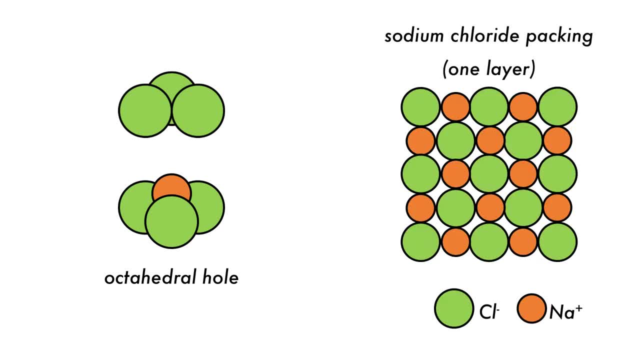 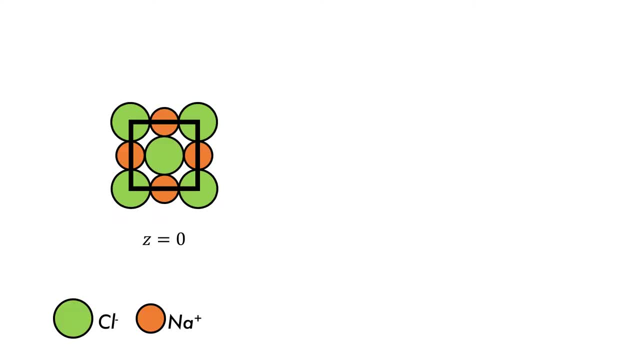 sodium chloride. The larger chloride ions create the octahedral holes for the smaller sodium ions. The sodium chloride structure can be viewed as an expanded FCC lattice. Here the chloride ions occupy large octahedral holes. This arrangement of ions gives the sodium ion as well as the 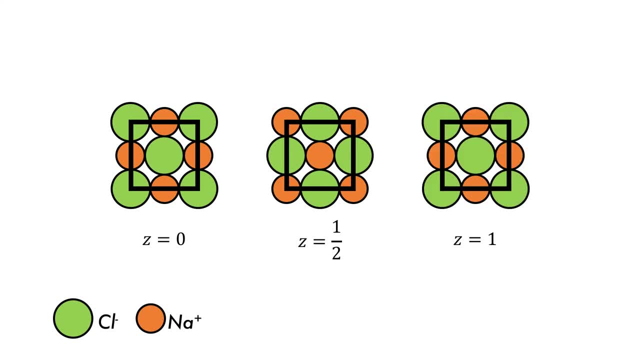 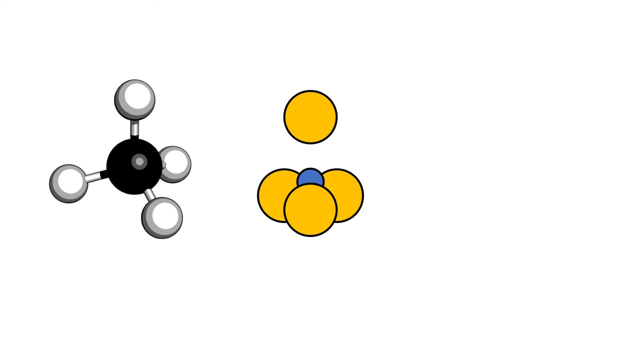 chloride ion, a coordination number of six. Each unit cell thus contains four sodium and four chloride ions with the stoichiometry NaCl. The next hole is the tetrahedral hole. The classic tetrahedral molecule is methane, with four equally spaced hydrogen atoms, A particle occupying a. 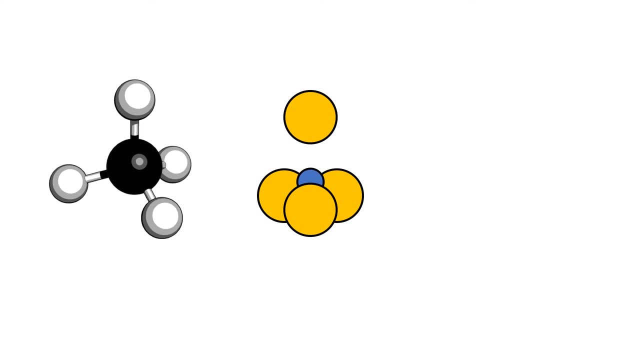 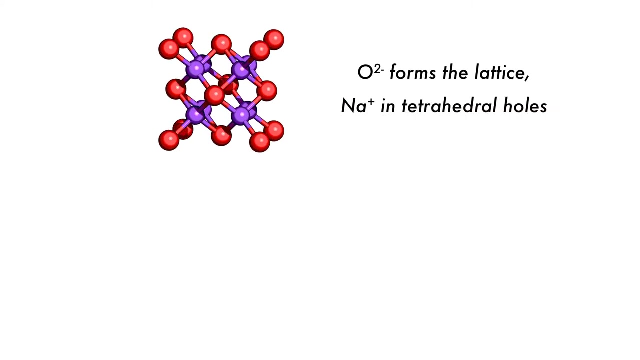 tetrahedral hole also has a coordination number of four. much like the carbon in methane, Tetrahedral holes tend to be smaller than octahedral holes. An FCC lattice has eight tetrahedral holes and four octahedral holes. Sodium oxide is a good example of an FCC-like lattice with sodium ions occupying the tetrahedral.